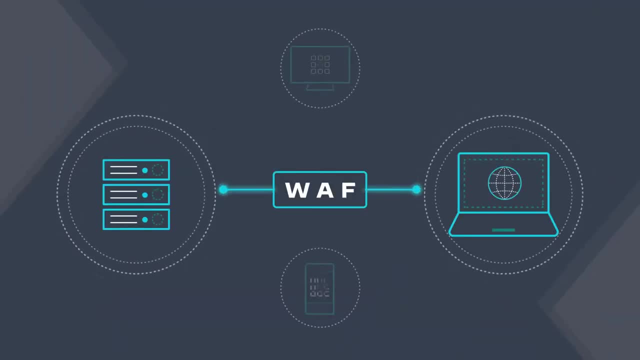 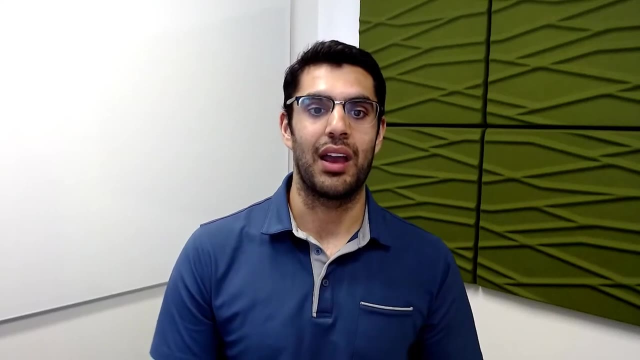 The key point I want to iterate again is that WAFs protect web applications from web-based attacks from the internet. Think of this as a bouncer at a nightclub who has to make sure that everyone in line has the right identification and is of the right age to determine if they 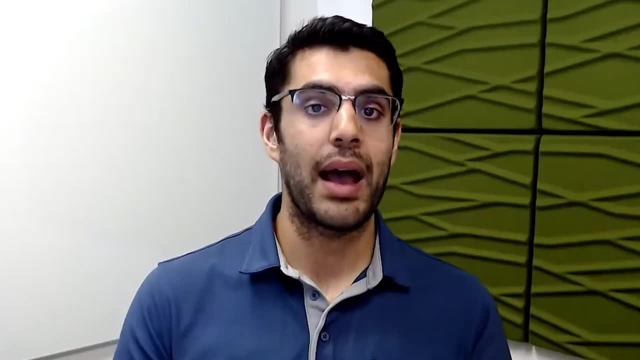 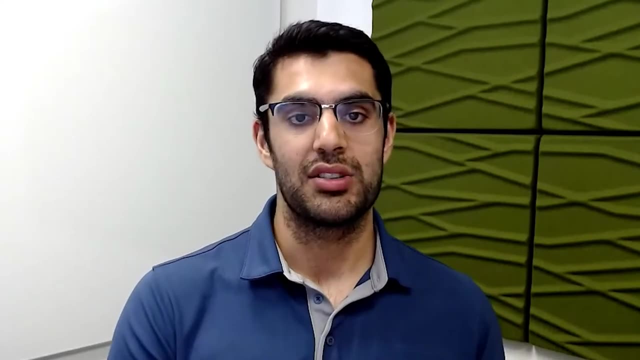 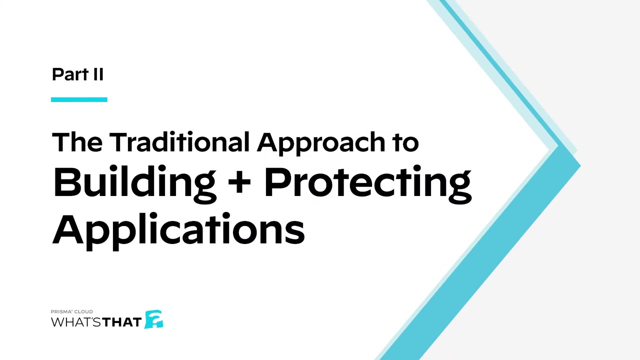 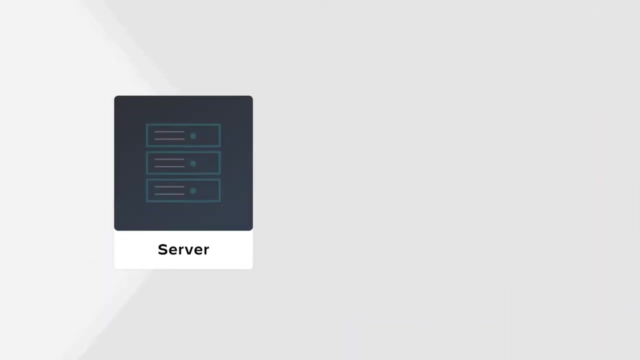 should be allowed into the club or not. Web app firewalls work very similarly. They protect the traffic to and from the internet with additional contact to determine if it should be allowed or denied. In the past, web applications were hosted from one physical server. A server was usually placed in your private data. 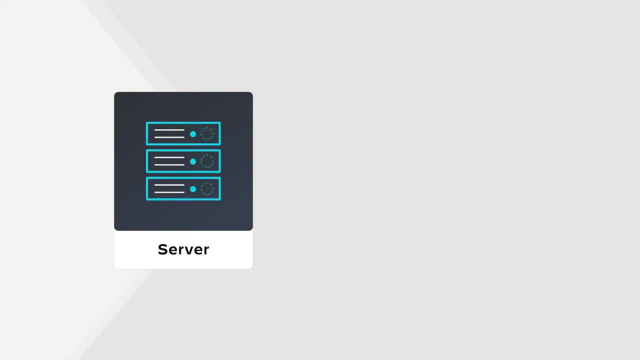 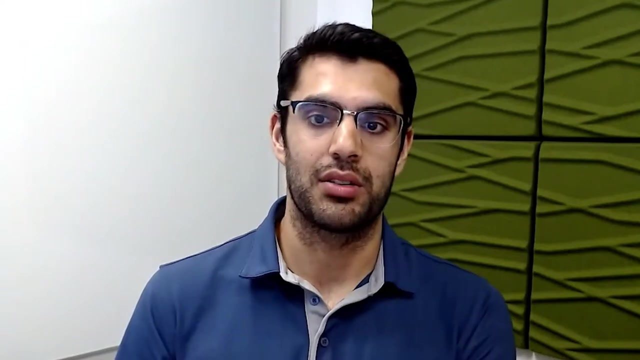 center within your network. All of the components of the web application- the web server, the application logic and the back-end database- were all in one place, So the perimeter of your web was very well defined. it was just a traffic to and from that server that you have to monitor. 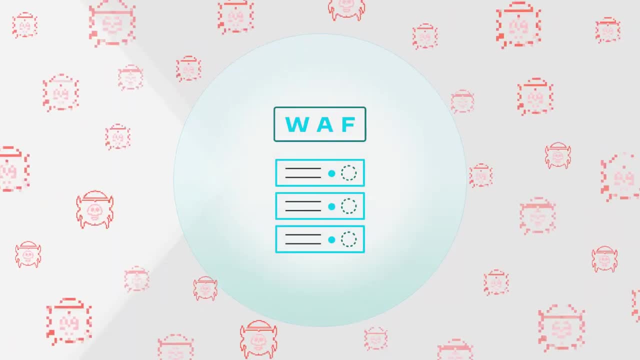 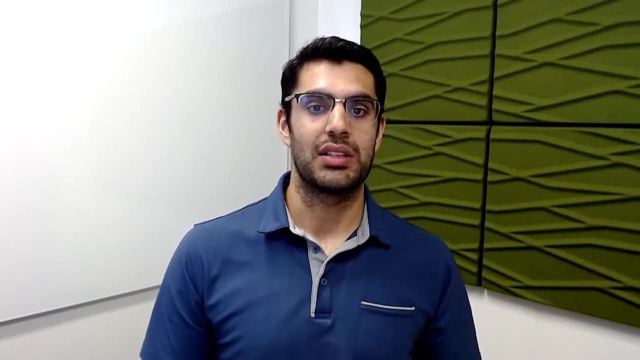 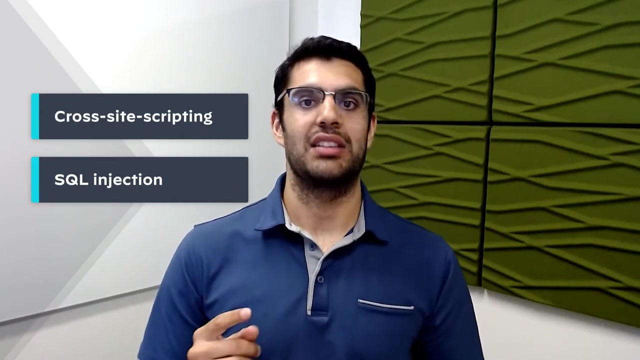 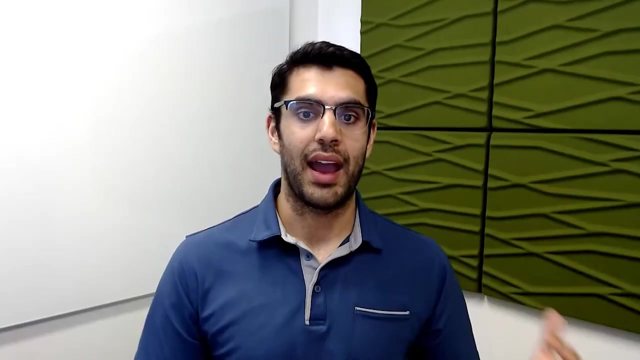 inspect now. this made it easy for you to place a web app firewall in front of your server to protect against web-based attacks. now these WAFs use policies to protect your applications from vulnerabilities and attacks like cross-site scripting, SQL injection, broken access control, and all of these attacks, if successful, would have given hackers access to the web application. 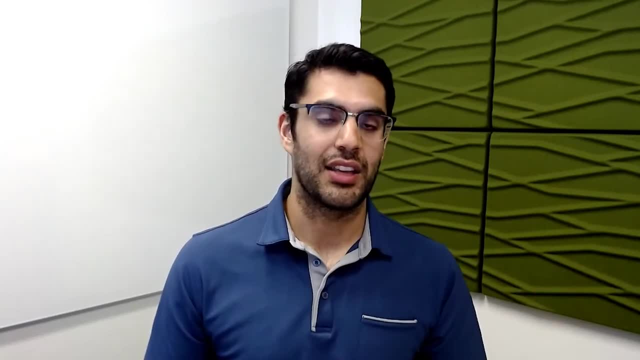 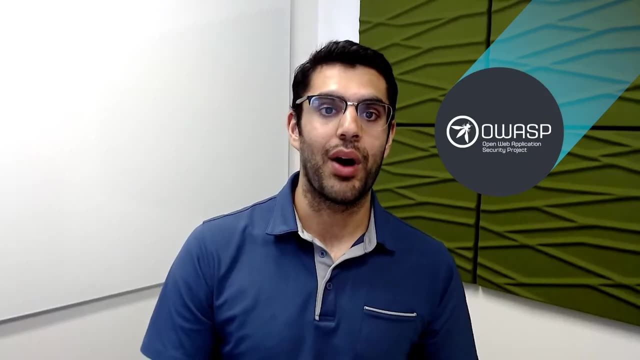 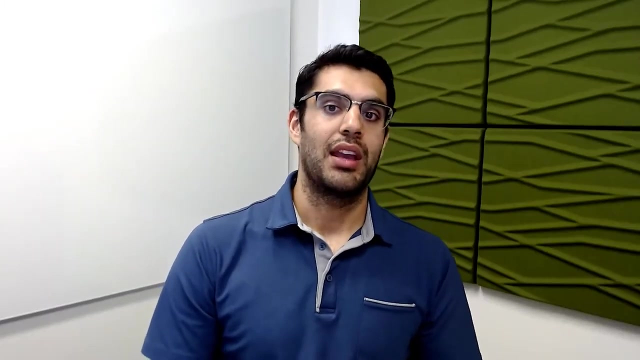 and the backup database clearly things that they should not have access to. the WAF was able to protect your application from these attacks, as well as attacks included in the OWASP top 10.. today, many organizations are moving their applications and data to the cloud using 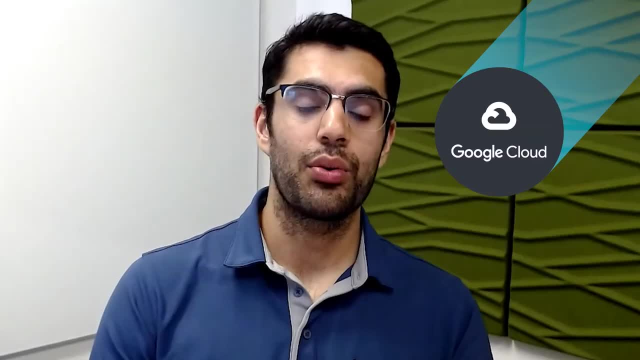 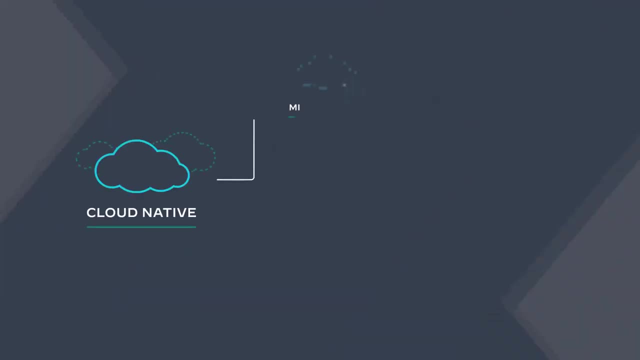 cloud products like AWS, Azure and GCP. more recently, companies have started developing their applications with the mindset of making them cloud native, by breaking up applications into microservices using containers and kubernetes. in fact, the cloud native computing Foundation found that 96 of organizations are either using or 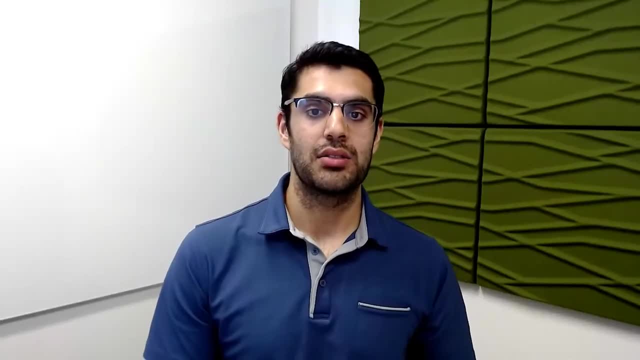 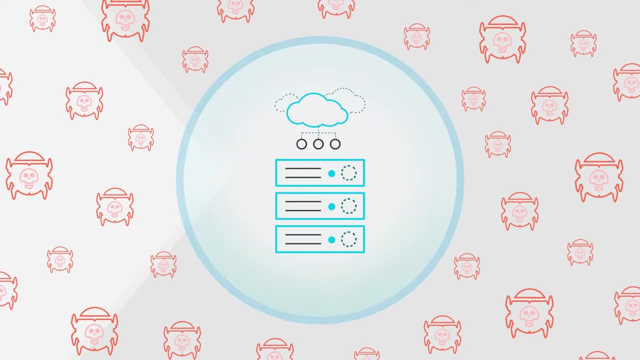 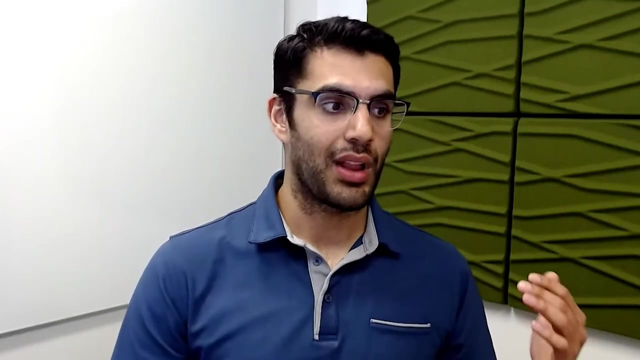 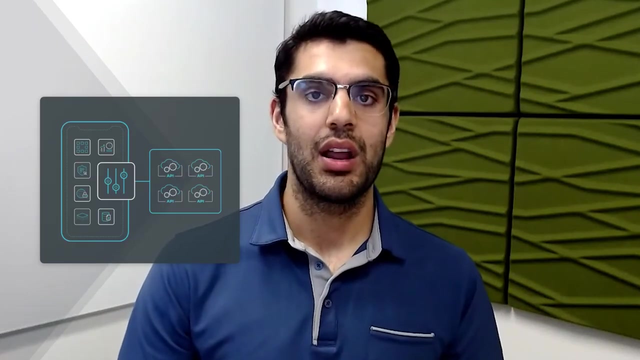 evaluating kubernetes. now, since these applications are built on different architectures, like containers, microservices and leveraging APIs, the legacy WAP is no longer sufficient to protect these types of applications. a lot of these applications even rely heavily on APIs to communicate, which adds another layer of complexity, making it even tougher to protect against.